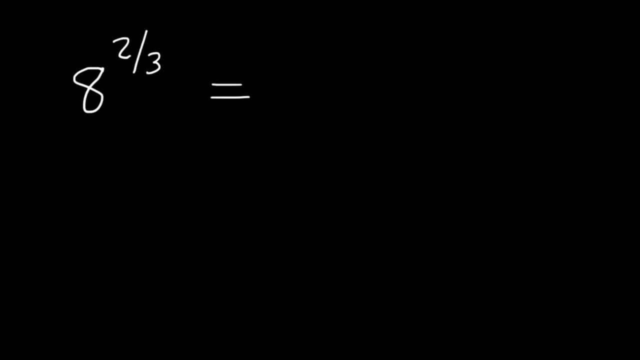 Now the best way to answer it is to separate the fraction into two parts. So this is equivalent to 8 raised to the 1 third power, which is raised to the second power. 1 third times 2 is 2 thirds. So what is 8 raised to the 1 third? Whenever you raise something to the 1 third power, 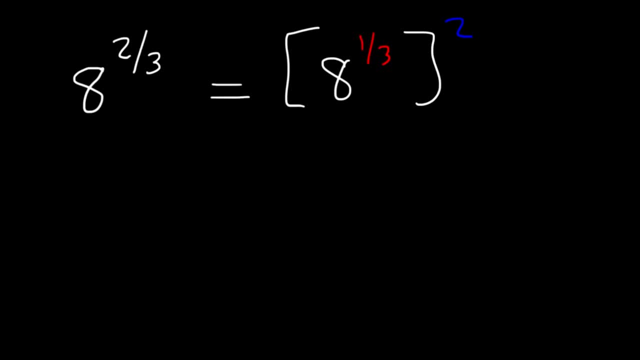 you're basically looking for the cube root. So what is the cube root of 8?? What number times itself? 3 times is 8.. So what times? what times? what is 8?? It turns out that the cube root of 8 is 2.. 2 times 2 times 2, 3 times is 8.. And so now we've got to figure out what 2 squared is. 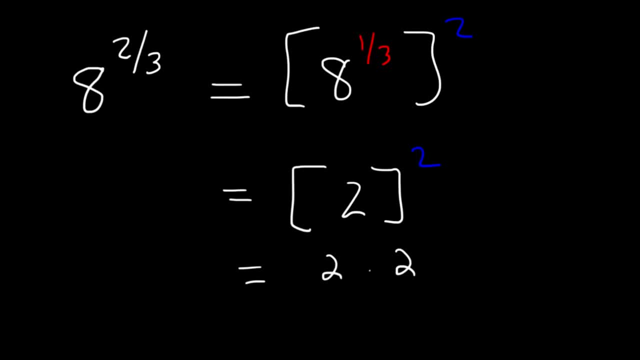 2 squared is basically taking two 2's and multiplying them together, 2 squared is equal to 4.. And so 8 is raised to the 2 thirds. power is 4.. So now that you know how to do that one, go ahead and try this one. 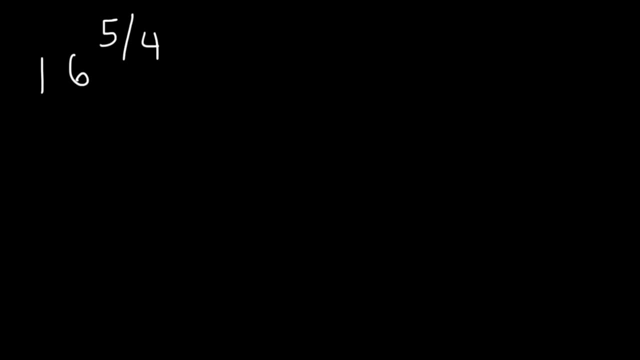 Calculate the value of 16 raised to the 5 fourths. So first let's find the 4th root of 16. And then let's raise it to the 5th power. So what number times itself? 4 times is equal to 16?. 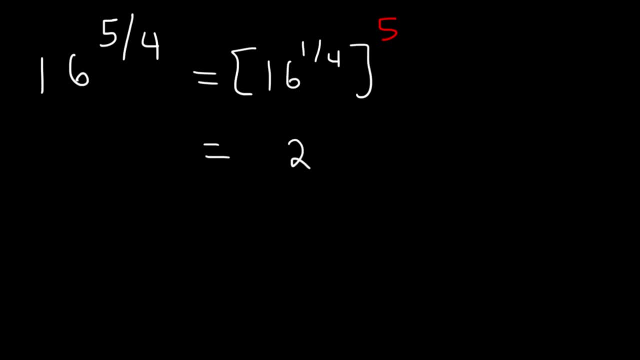 The 4th root of 16 is 4.. So what number times itself 4 times is 2? Because 2 times 2 times, 2 times 2, 4 times is 16.. Now what is the value of 2 to the 5th power? 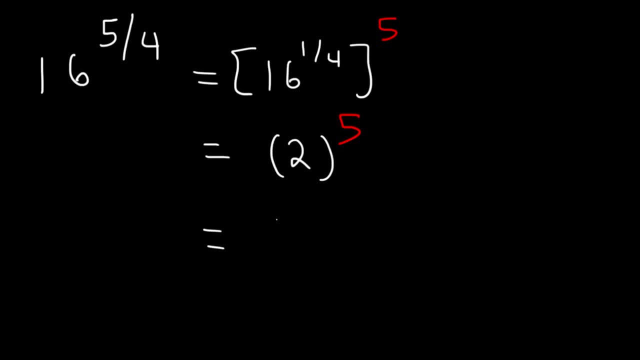 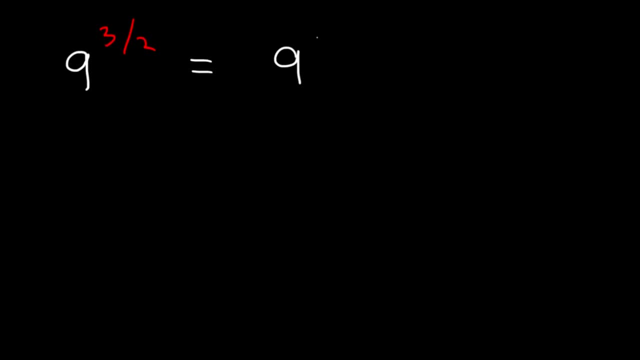 So once again, we're going to find the square root of 9,, which is 9 to the 1 half, and then we're going to raise it to the 3rd power. The square root of 9 is 3.. 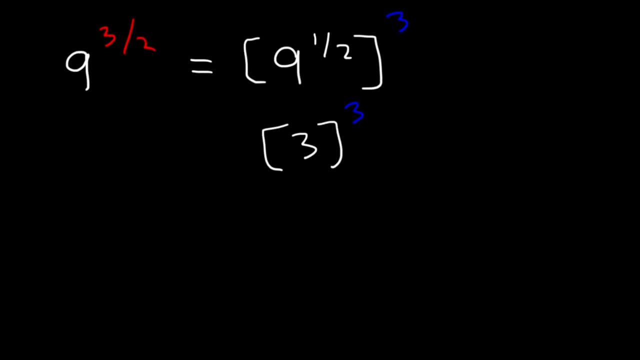 And 3 to the 3rd power, which is basically 3 times 3 times 3. 3 times 3 times 3 is 9.. 9 times 3 is 27.. So 9 to the 3 halves is 27.. 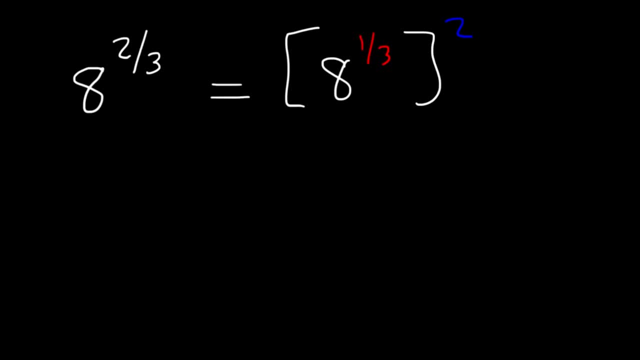 you're basically looking for the cube root. So what is the cube root of 8?? What number times itself? 3 times is 8.. So what times? what times? what is 8?? It turns out that the cube root of 8 is 2.. 2 times 2 times 2, 3 times is 8.. And so now we've got to figure out what 2 squared is. 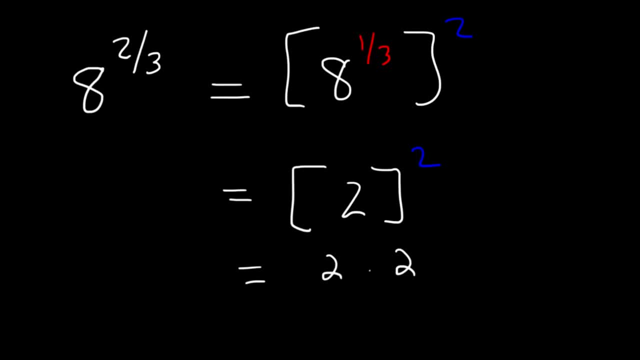 2 squared is basically taking two 2's and multiplying them together, 2 squared is equal to 4.. And so 8 is raised to the 2 thirds. power is 4.. So now that you know how to do that one, go ahead and try this one. 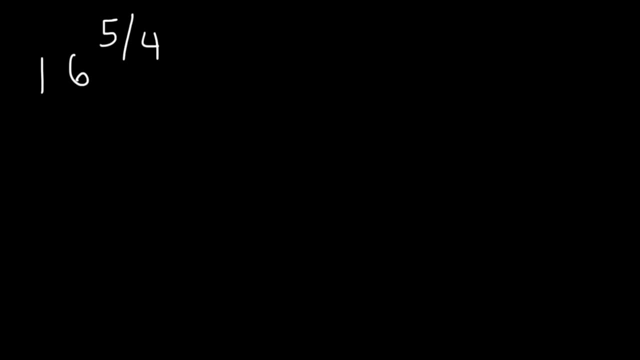 Calculate the value of 16 raised to the 5 fourths. So first let's find the 4th root of 16. And then let's raise it to the 5th power. So what number times itself? 4 times is equal to 16?. 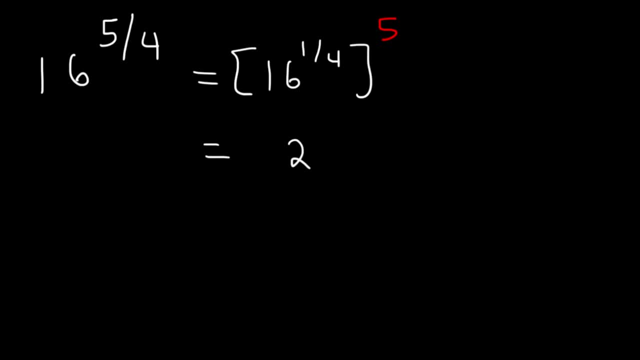 The 4th root of 16 is 4.. So what number times itself 4 times is 2? Because 2 times 2 times, 2 times 2, 4 times is 16.. Now what is the value of 2 to the 5th power? 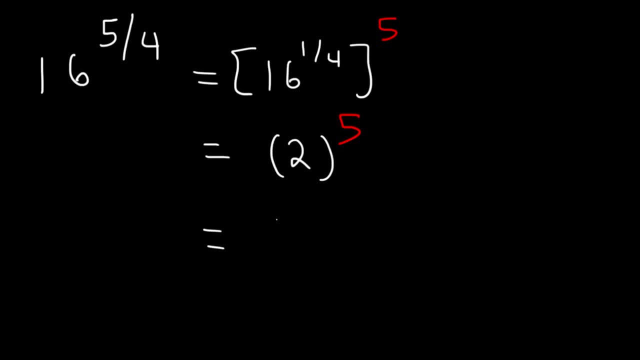 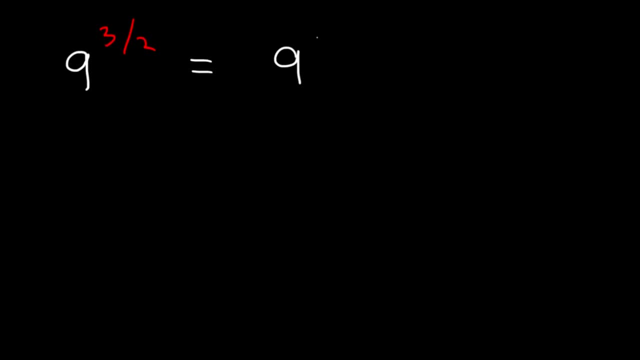 So once again, we're going to find the square root of 9,, which is 9 to the 1 half, and then we're going to raise it to the 3rd power. The square root of 9 is 3.. 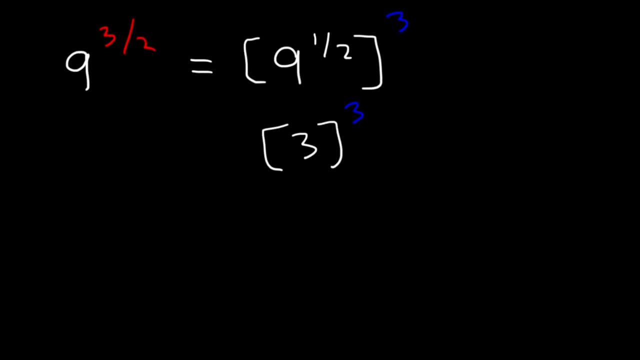 And 3 to the 3rd power, which is basically 3 times 3 times 3. 3 times 3 times 3 is 9.. 9 times 3 is 27.. So 9 to the 3 halves is 27.. 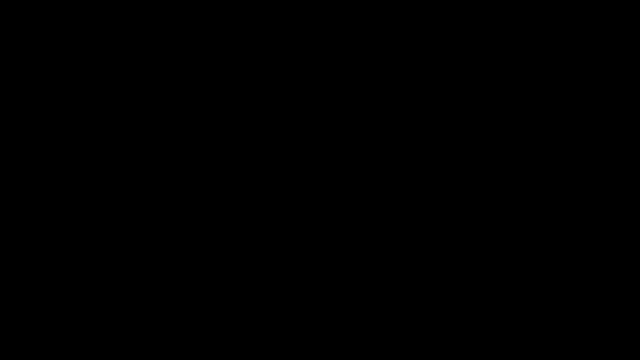 So 9 to the 3 halves is 27.. So now we're going to do the same thing with the cube root of 64.. So now we're going to do the same exercise. What is the cube root of 64 squared? 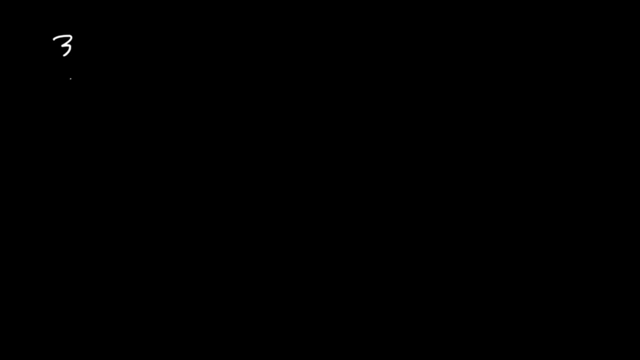 So 2 times 4 plus 4 times 2, which is 6 to the 3 thirds. What is the cube root of 64 squared? So what we can do if we have a radical and an exponent on the inside, What we can do is, well, you can change it into its exponential form. 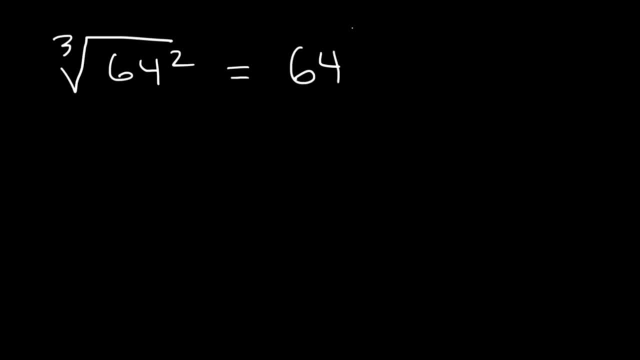 You can write it as a fractional exponent. This is equivalent to 64 raised to the 2 3rds, which is the cube root of 64 raised to the 2nd power. So what is the error? Well, the error is 1.. 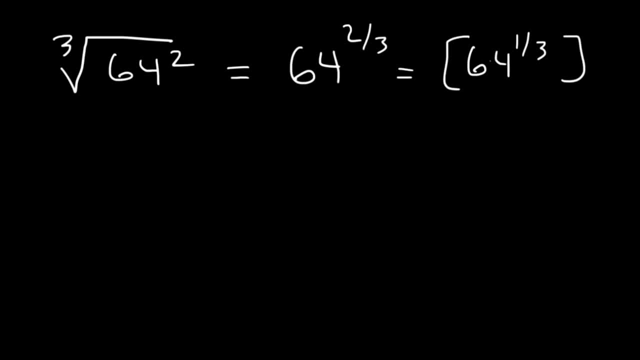 second power. Now, what is the cube root of 64?? What number times itself three times is 64? 4 times 4 times 4, that's 64. So we're going to have 4 squared, and 4 squared, or 4 times 4, is 16.. So the cube root of 64 squared is simply 16.. Try this. 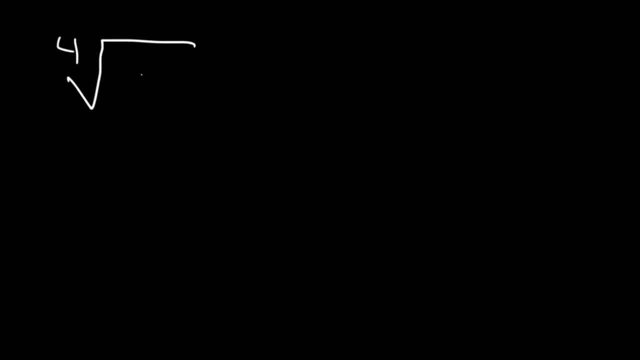 one Calculate the 4th root of 81 cubed, So let's rewrite it. This is 81 raised to the 3 4ths, which we can find the 4th root first, and then we'll raise it to the 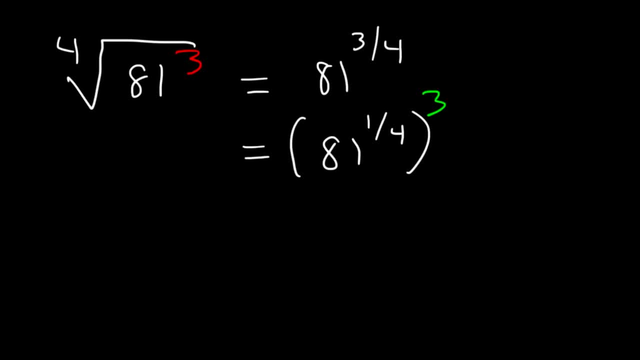 third power: The 4th root of 81 is 3, because 3 times 3 times, 3 times 3, 4 times is 81. And 3 to the 3rd. we've calculated this value already: it's 27.. Here's another one. 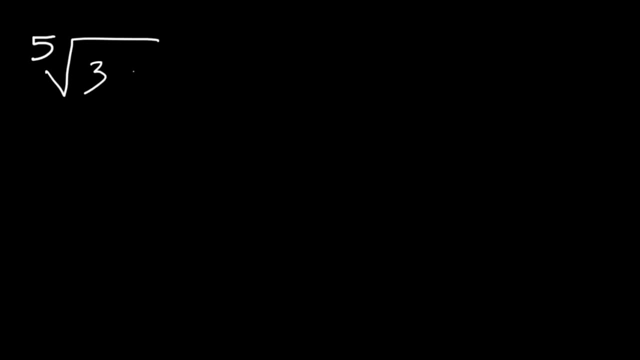 that we could try. What about the 5th root of 32 raised to the 4th power? So, just like before, we can rewrite it like this: So we need to find the 5th root first and then raise it to the 4th power. 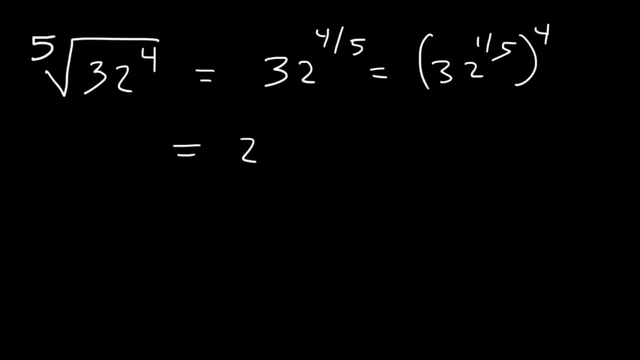 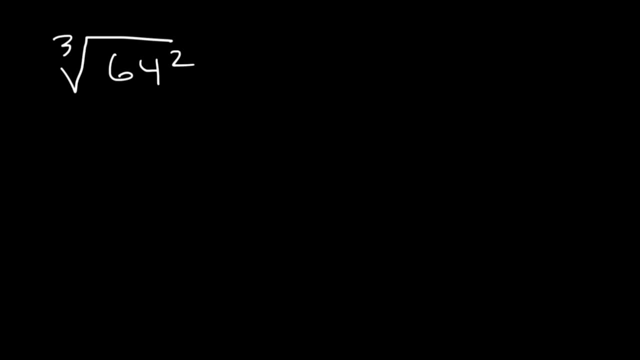 What can we do if we have a radical and an exponent on the inside? Well, you can change it into its exponential form. you can write it as the fractional exponent. This is equivalent to 64 raised to the 2 thirds, which is the cube root of 64. 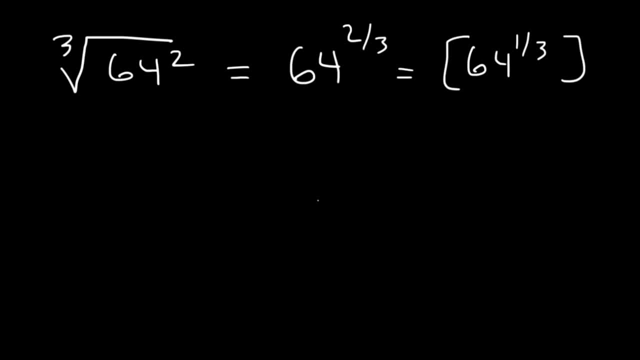 raised to the 2nd power. second power Now, what is the cube root of 64?? What number times itself three times is 64? 4 times 4 times 4, that's 64. So we're going to have 4 squared and 4. 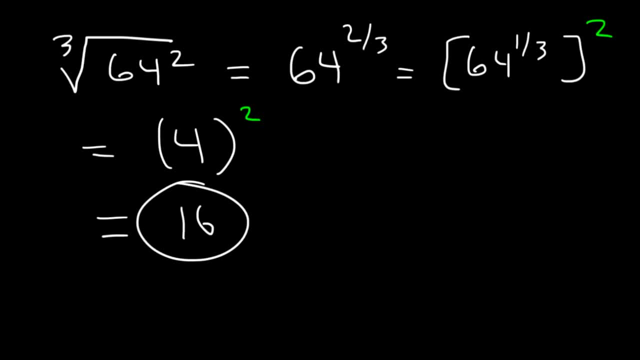 squared, or 4 times 4, is 16.. So the cube root of 64 squared is simply 16.. Try this one: Calculate the fourth root of 81 cubed. So let's rewrite it. This is 81 raised to the 3 fourths which we can find the fourth root first, and then we'll 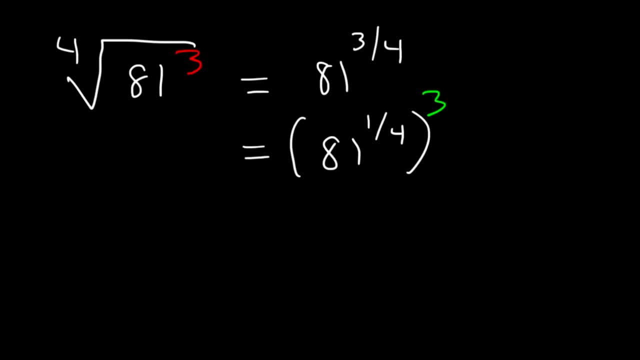 raise it to the third power. The fourth root of 81 is 3, because 3 times 3 times, 3 times 3, 4 times is 81. And 3 to the third. we've calculated this value already: it's 27.. Here's another one. 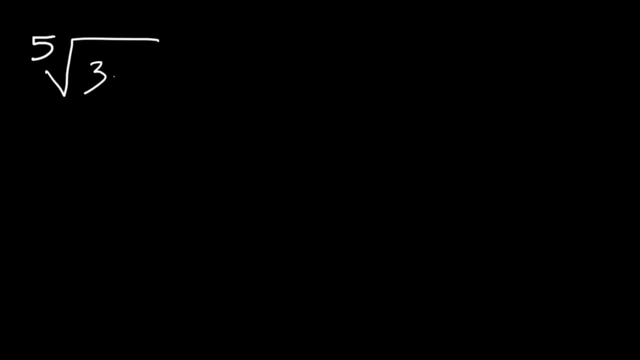 that we could try. What about the fifth root of 32 raised to the fourth power? So, just like before, we can rewrite it like this: So we need to find the fifth root first and then raise it to the fourth power. The fifth root of 32 is 5, I mean not 5, but 2.. And 2 to the fourth power, that's 2. 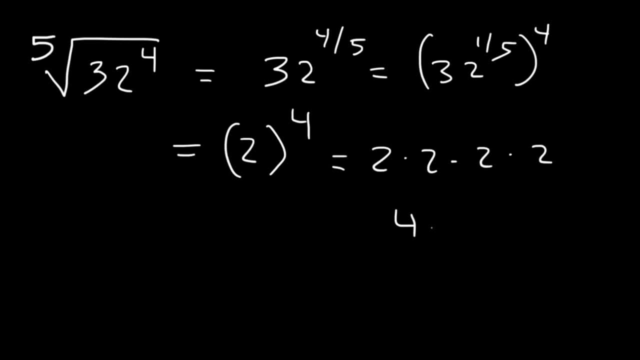 times 2 times 2 times 2.. 2 times 2 is 4, and those 2's will also make a 4.. 4 times 4 is 16.. So 16 is the final answer. Now, what would you do if we have a negative exponent? 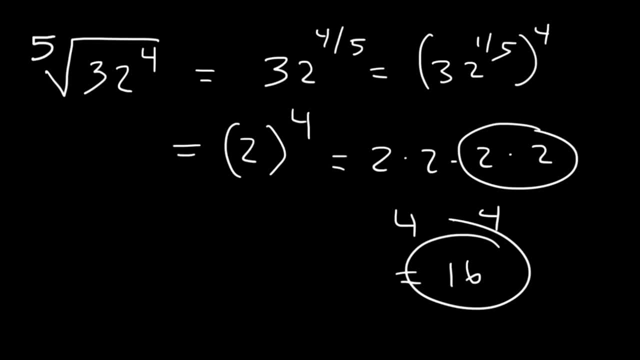 16.. So 16 is the final answer. Now, what would you do if we have a negative exponent? Let's say 25 raised to the 3rd power, 3 over 2. What does that equal? If you have a negative exponent, you can make it positive. 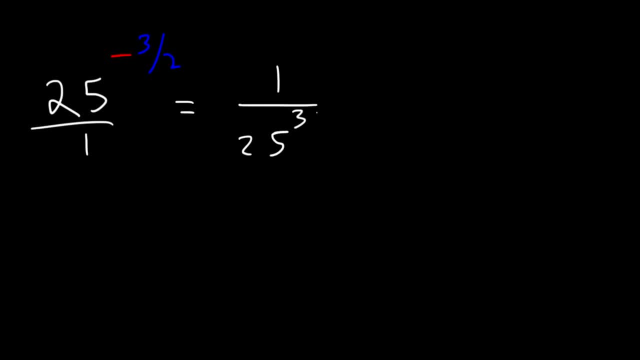 by taking the 25 and putting it to the bottom. Now, first we need to find the square root of 25, and then we need to raise it to the third power. The square root of 25 is 5, and if we raise it to the third power 5 times, 5 times 5,, 3 times, that's 125.. So the final. 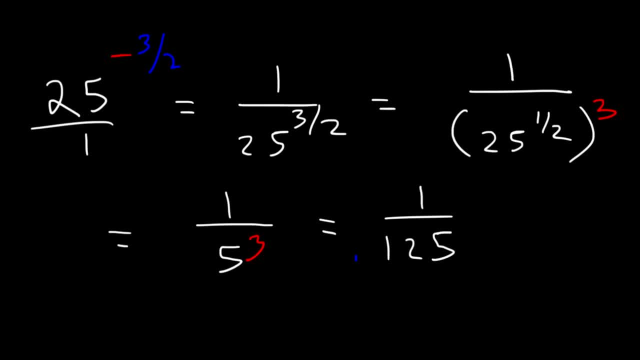 answer is 1 divided by 125, and so that's it. Now, how would you simplify this expression? What is the cube root of x to the fourth power multiplied by the fourth root of x to the fifth power? What would you do here? Now, we can't multiply x. 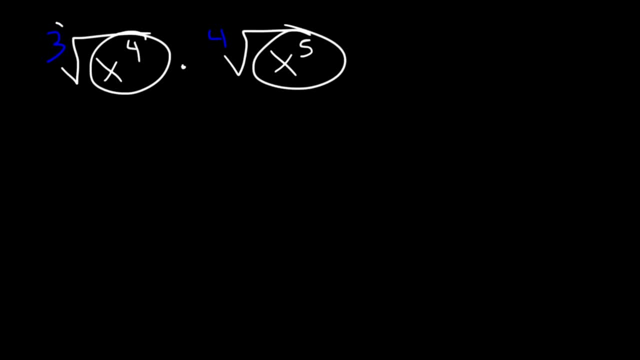 to the fourth times x to the fifth. the reason being is: the index numbers are not the same. If they were the same, we could do that, but since they're not the same, we can't. So how can we simplify this expression? In order to do so, we need to convert the radical expression. 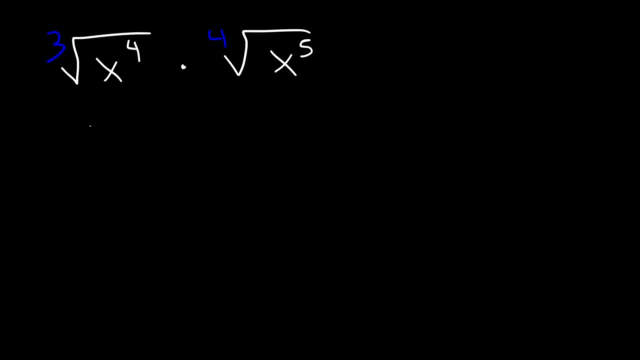 to a fractional exponent. So the cube root of x to the fourth is the same as x raised to the four thirds, and the other one is going to be x raised to the five fourths. Now let's go over some basic rules of algebra. Whenever you multiply by a common base, you may add the exponents, So x squared. 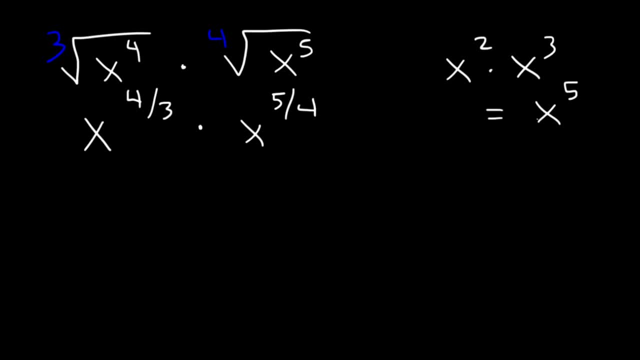 times x. cubed is x to the fifth power. 2 plus 3 is 5.. So in this case we need to add the two fractions and to add them you need to get common denominators. So let's find out what 4 over 3 plus 5 over 4 is equal to The least common multiple of. 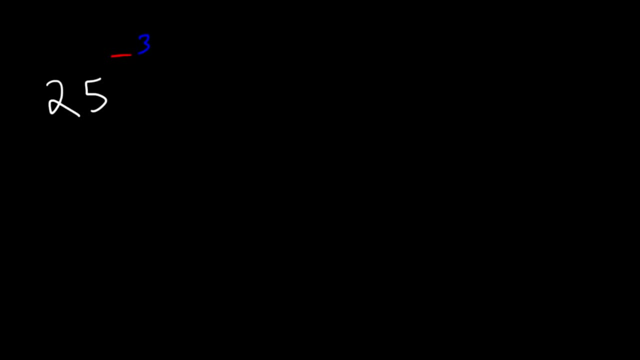 Let's say 25 raised to the 3rd power, 3 over 2.. What does that equal? If you have a negative exponent, you can make it positive by taking the 25 and putting it to the bottom. Now, first we need to find: 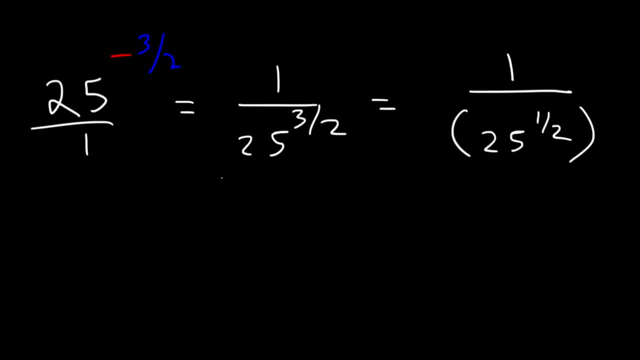 the square root of 25, and then we need to raise it to the third power. The square root of 25 is 5.. And 5 raised to the third power 5 times, 5 times 5, 3 times that's 125. So the final answer is 1 divided by 125.. And so that's it. Now how? 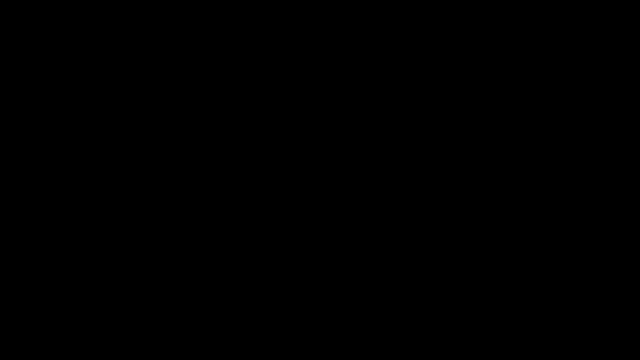 would you simplify this expression? What is the cube root of x to the fourth power multiplied by the fourth root of x to the fifth power? What would you do here? Now, we can't multiply x to the fourth times x to the fifth. The reason being is the index numbers are not the same If they. 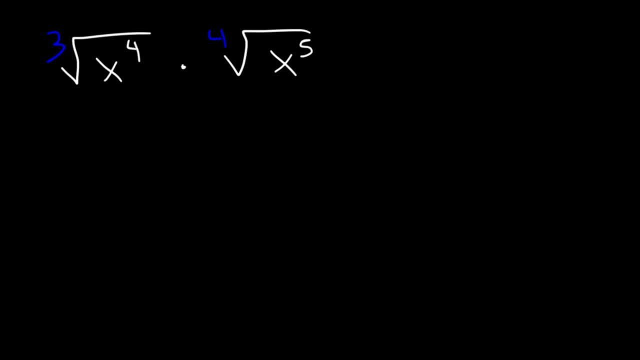 were the same, we could do that, But since they're not the same, we can't. So how can we simplify this expression? In order to do so, we need to convert the radical expression to a fractional exponent, So the cube root of x to the fourth is the same as the square. 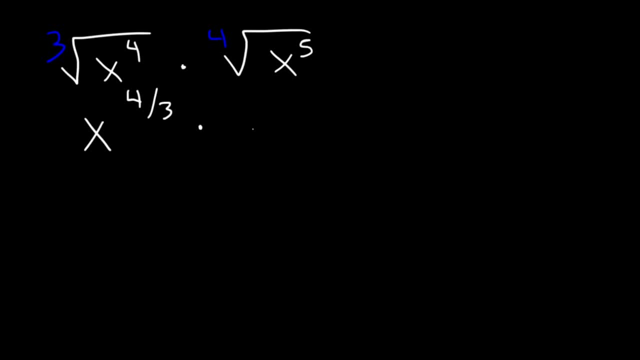 root of x raised to the fourth And the other one is going to be x raised to the fifth. Now let's go over some basic rules of algebra. Whenever you multiply by a common base, you may add the exponents. So x squared times, x cubed is x to the fifth, power 2 plus 3. 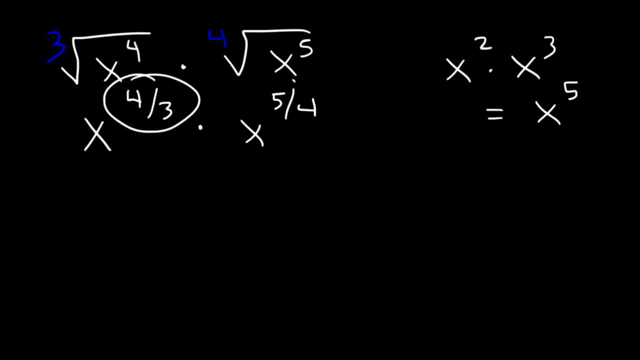 is 5.. So in this case we need to add the two fractions, And to add them you need to get common denominators. So let's find out what 4 over 3 is. 1 plus 5 over 4 is equal to The least common multiple of 3 and 4 is 12.. So let's multiply. 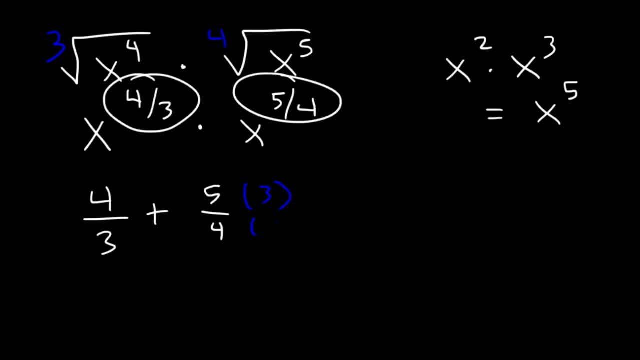 3 and 4 is 12.. So let's multiply this fraction by 3 over 3, and the other one by 4 over 4.. So this is going to equal 16 over 12, plus 15 over 12.. 16 plus 15 is 31.. So this is going. 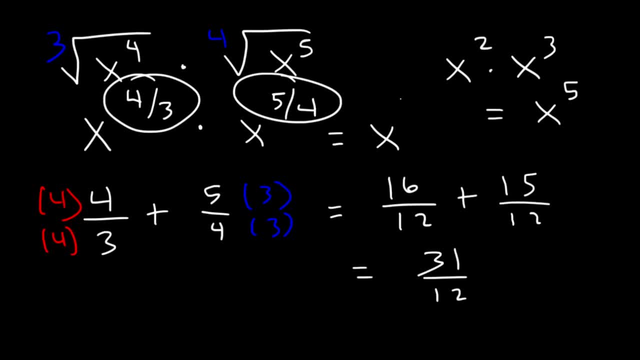 to equal 31 over 12.. So thus we have x raised to the 31 over 12, which we can rewrite it as the 12th root of x to the 31 power. Now, if we want to, we can simplify that radical. It's not fully simplified, but let's go ahead. 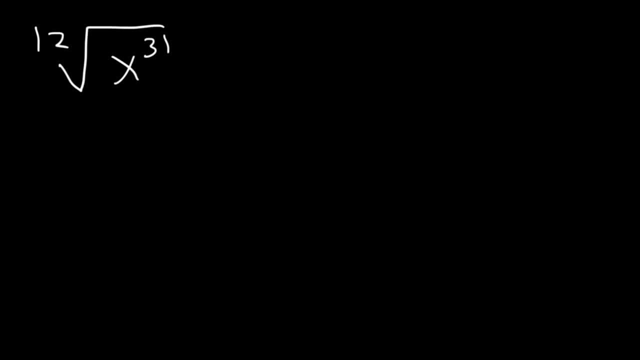 and simplify it. Now, how many times does 12 go into 31?? 12 goes into 31 two times. So this is going to equal 31 two times Twelve times 2 is 24, but first I'm going to split it into two radicals. 24 and 7 adds. 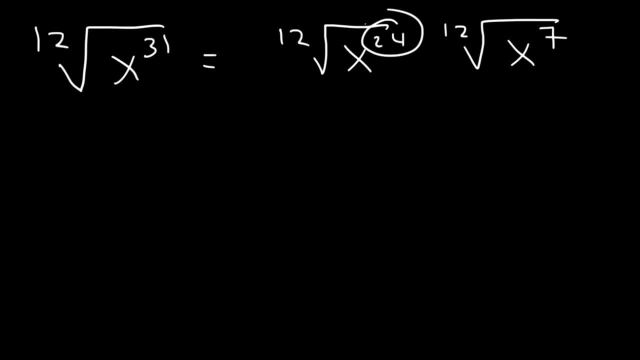 up to 31.. Now, 24 divided by 12 is 2, so this is going to be x squared times the 12th root of x to the 7.. So, if you want to simplify it, That's the final answer. 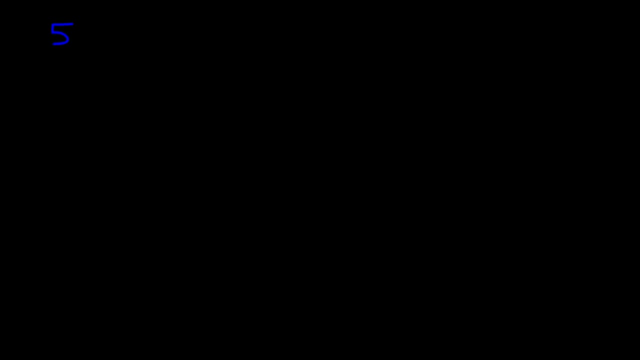 Let's try this one. What is the fifth root of x cubed divided by, let's say, the fourth root of x to the 7?? Try this one, Go ahead and simplify it. So, first let's convert it into a fractional exponent. This is going to be x raised to. 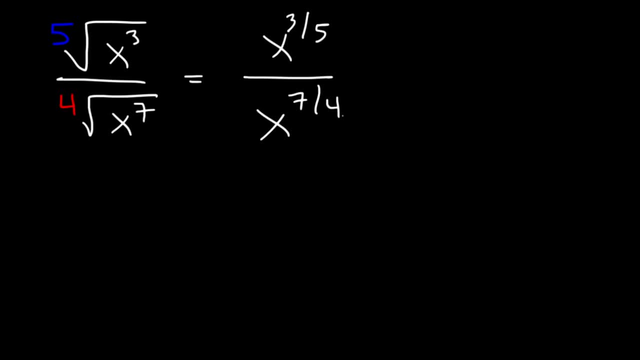 the 3 over 5.. divided by x, raised to the 7 over 4.. Now, when you're dividing by two common bases, you need to subtract the exponents. 7 minus 2 is 5.. So in this case we've got to subtract the fractions. 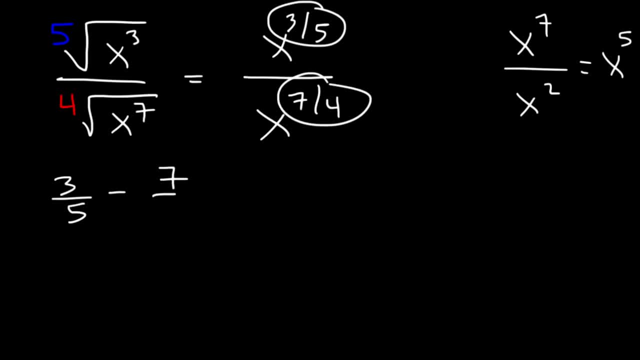 So we have 3 over 5, minus 7 over 4.. So let's go ahead and get common denominators. Let's multiply this fraction by 5 over 5, and the other one by 4 over 4.. So this will give us a common denominator of 20.. 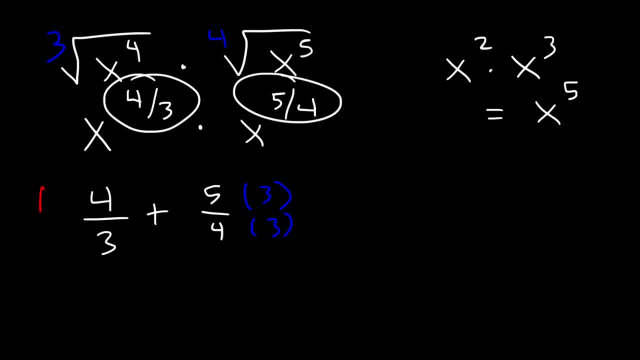 this fraction by 3 over 3 and the other one by 4 over 4.. So this is going to equal 16 over 12, plus 15 over 12.. 16 plus 15 is 31.. So this is 31 over 12.. So thus we have x. 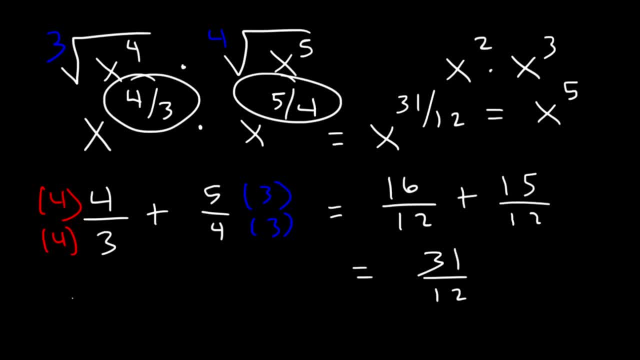 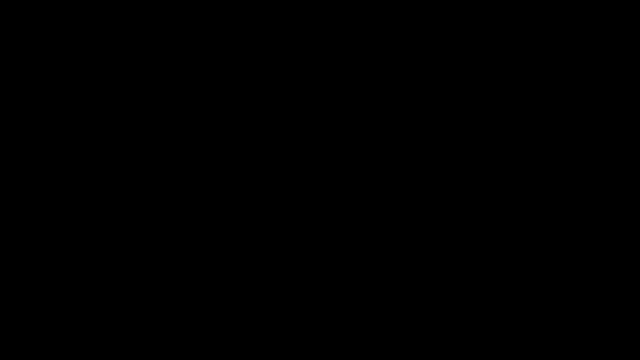 raised to the 31 over 12, which we can rewrite it as the 12th root of x to the 31 power. Now, if we want to, we can simplify that radical. It's not fully simplified, but let's go ahead. 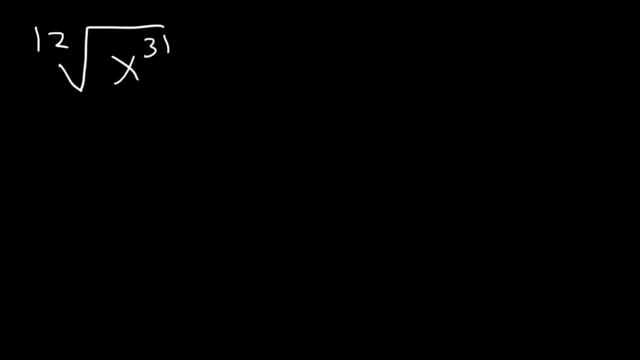 and simplify it Now, how many times does 12 go into 31? 12 goes into 31. two times 12 times 2 is 24.. But first I'm going to split it into two radicals. 24 and 7 adds. 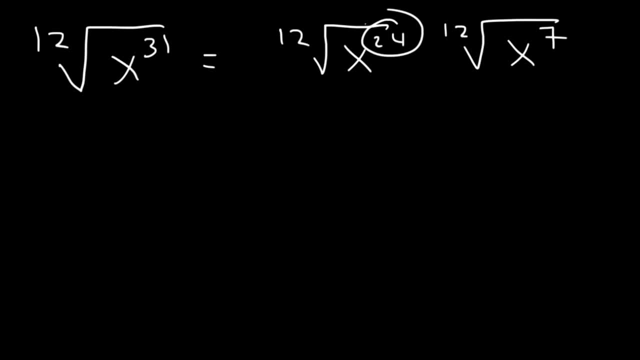 up to 31.. Now, 24 divided by 12 is 2.. So this is going to be x squared times the 12th root of x to the 7.. So, if you want to simplify it, that's the final answer. 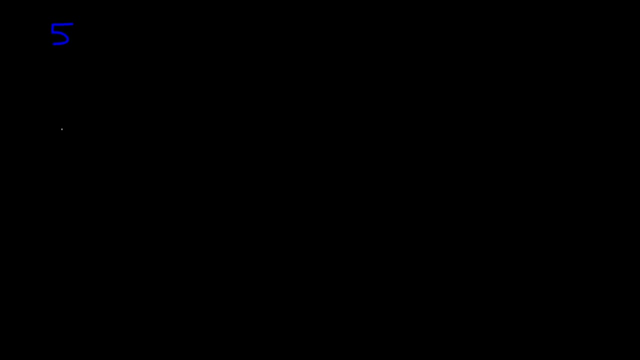 Let's try this one. What is the 5th root of x cubed divided by, let's say, the 4th root of x to the 7?? Try this one, Go ahead and simplify it. So first let's convert it into: 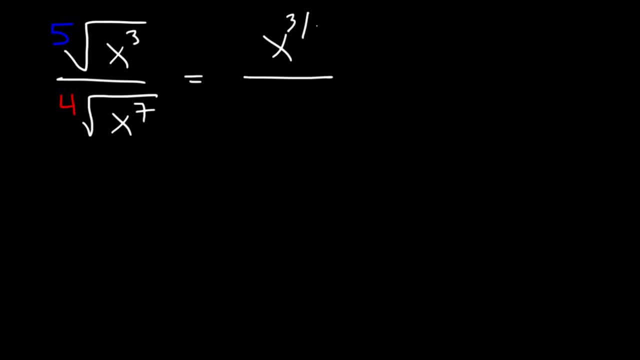 a fractional exponent. This is going to be x raised to the 3 over 5 divided by x raised to the 7 over 4.. 2 common bases: You need to subtract the exponent: 7 minus 2 is 5.. So in this case, 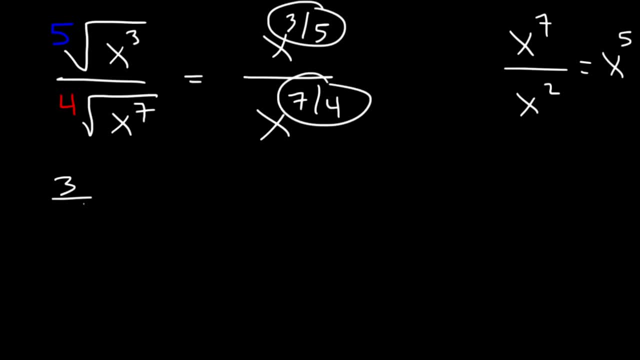 we've got to subtract the fractions, So we have 3 over 5 minus 7 over 4.. So let's go ahead and get common denominators. Let's multiply this fraction by 5 over 5 and the other one by 4 over 4.. So this will give us a common denominator of 20.. 4 times 3 is 12.. 4 times.